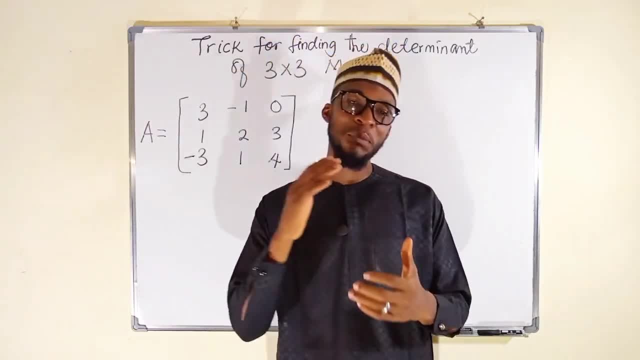 Hello good day viewers. In this tutorial, I am going to show you a simple trick to find the determinant of 3x3 matrix. So if you are new here consider subscribing. Press the bell 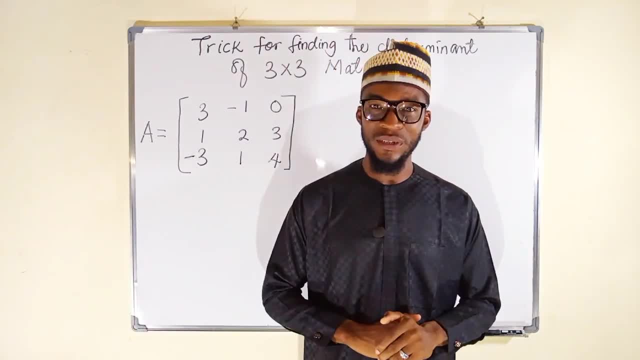 icon so that you will be notified whenever I upload a new content and don't forget to share to your learning colleagues. But before we start, I want to ask you this simple question. 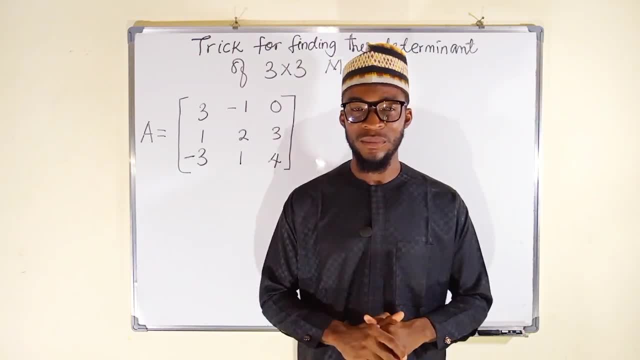 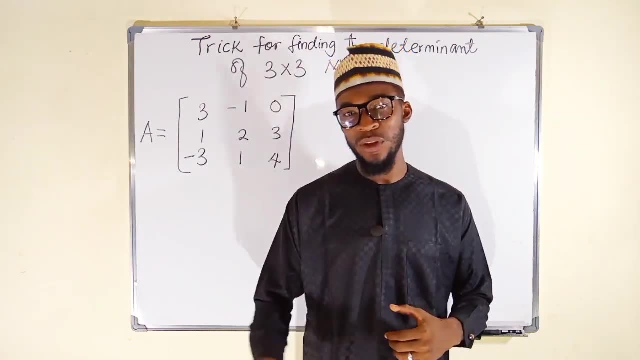 Thumbel mask class has over 9000 subscribers but I hardly gain 500 views per video. Kindly state the reason in the comment box below. So let's get started. You can see I have already 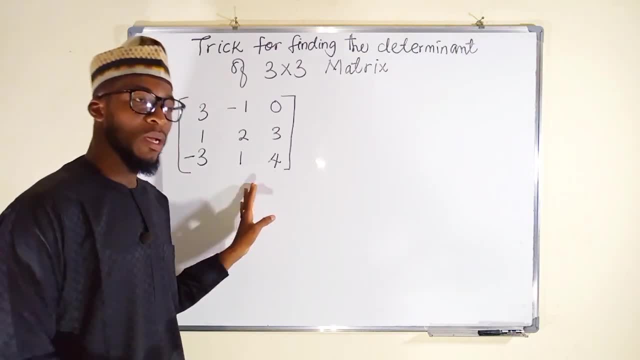 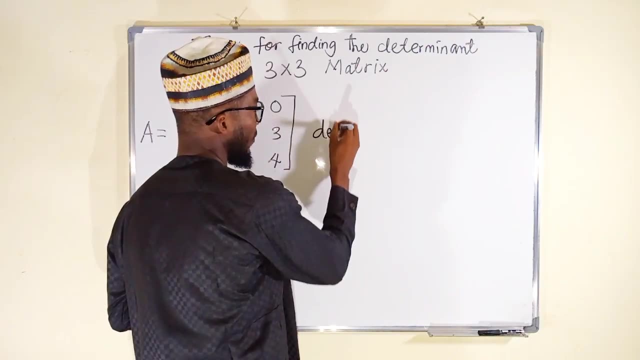 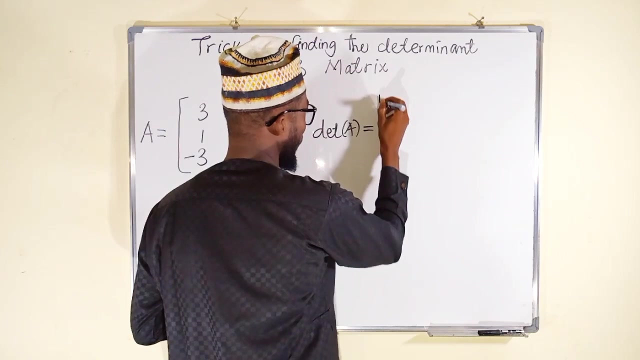 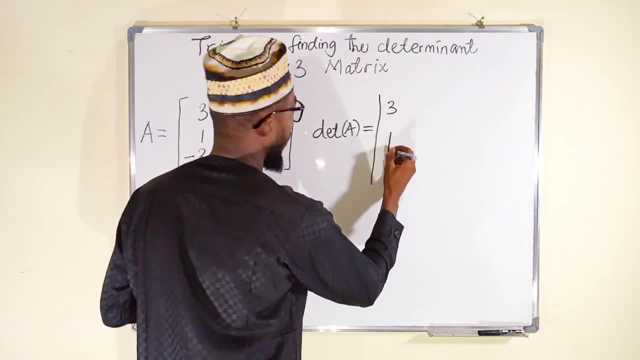 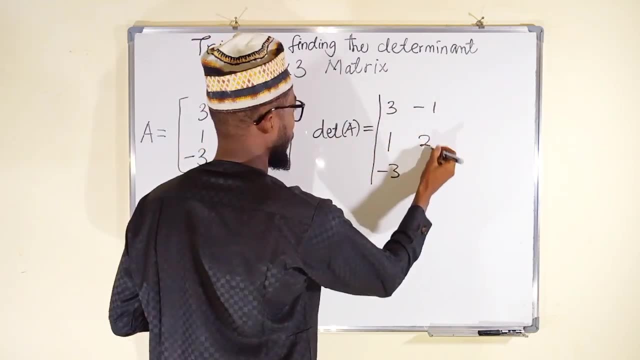 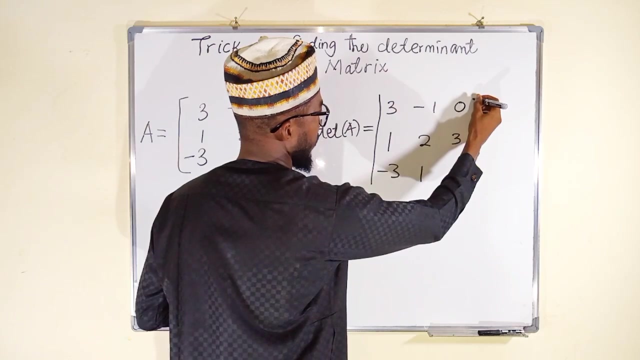 We have three, we have one, and we have negative three. The next one is negative one, two, and one. The last column we have zero, three, and four. Next, repeat the first and second 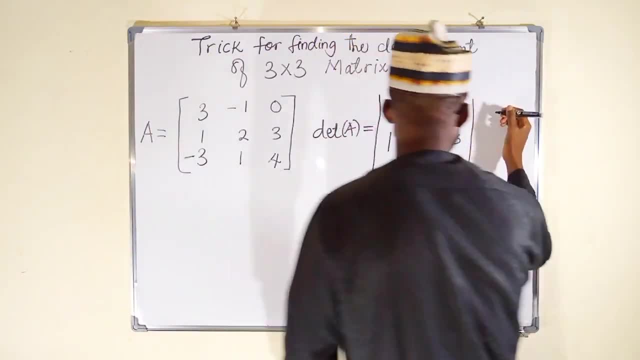 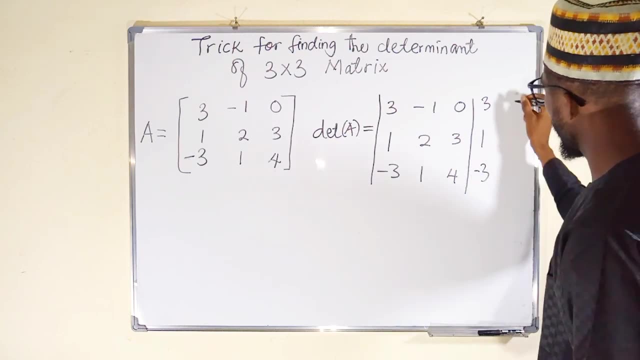 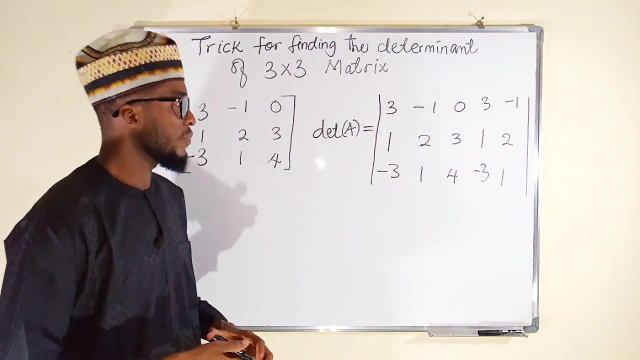 column. We have 3, 1, negative 3, negative 1, 2, and 1. Okay, let me even remove this one. Okay, what do we do next? We are going to take the product of this element diagonally 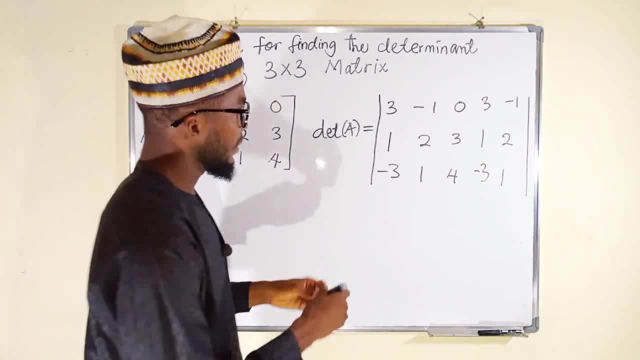 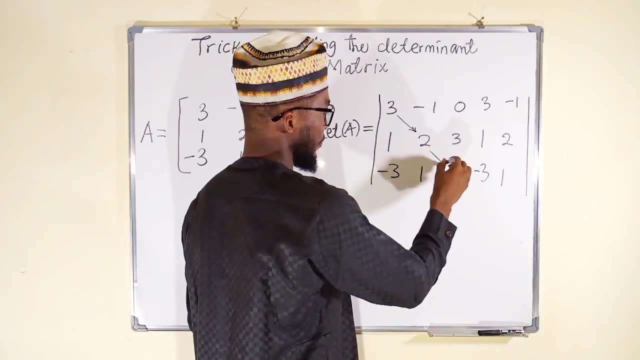 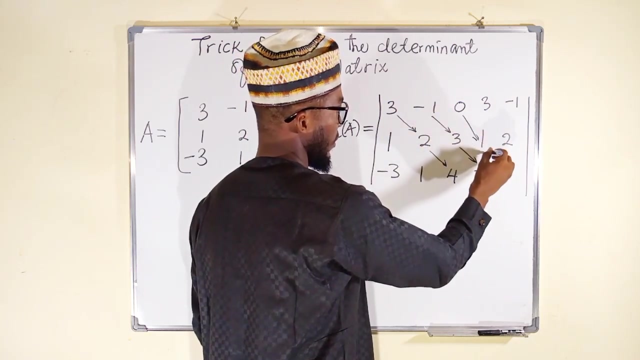 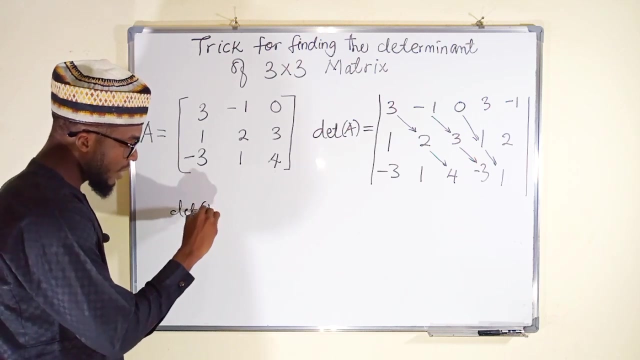 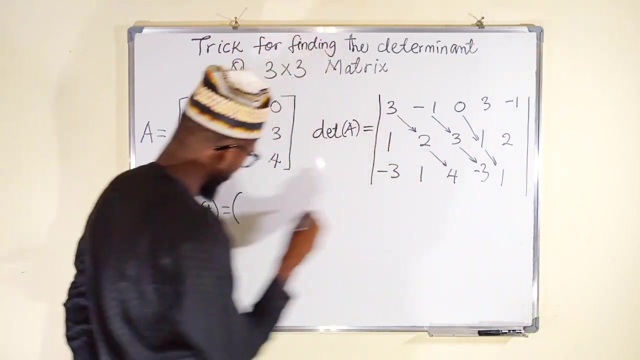 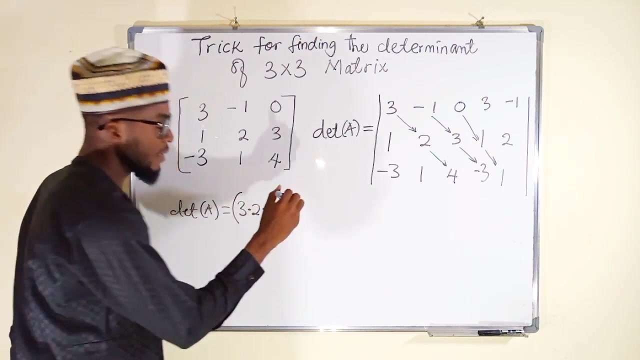 from the top left corner. So let's start with this one. Product. Okay, this is going to be a summation. And this is the last one. So to find the determinant, we say that the determinant of this matrix A will now be equal to, we multiply this. 3 times 2 times 4. 3 times 2 times 4. We close. We add again. Negative 1 times 3 times negative 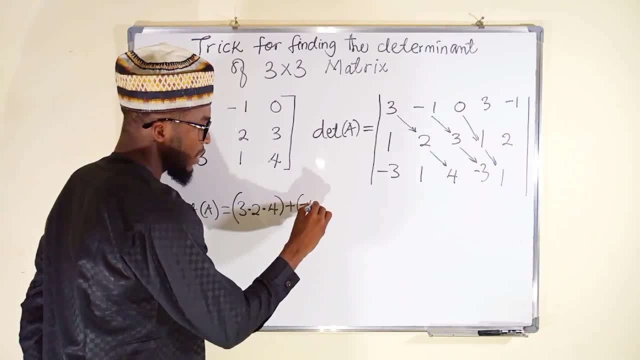 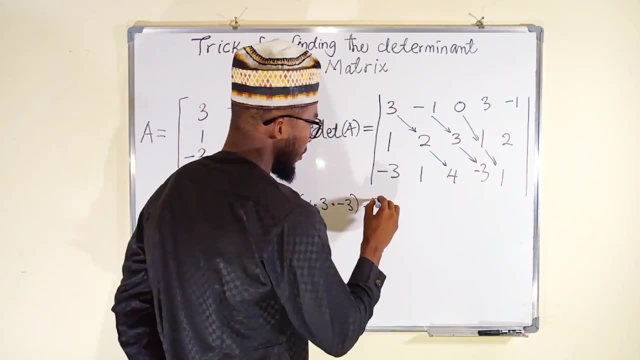 3. We have negative 1 multiplied by 3 multiplied by negative 3. Then we add again. 0 times 1 times 1. We have 0. 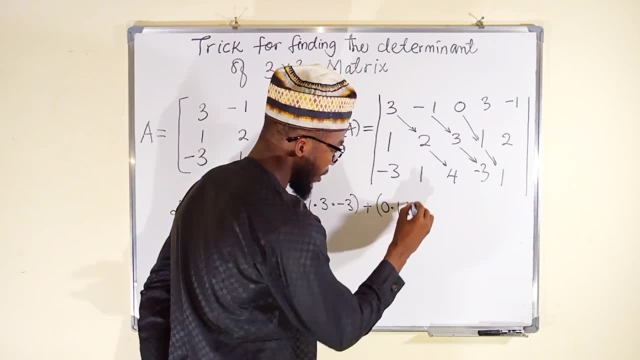 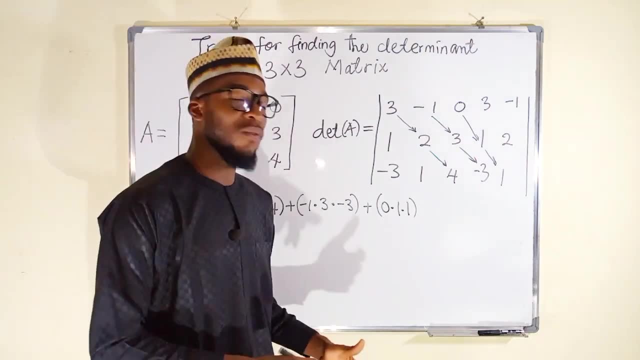 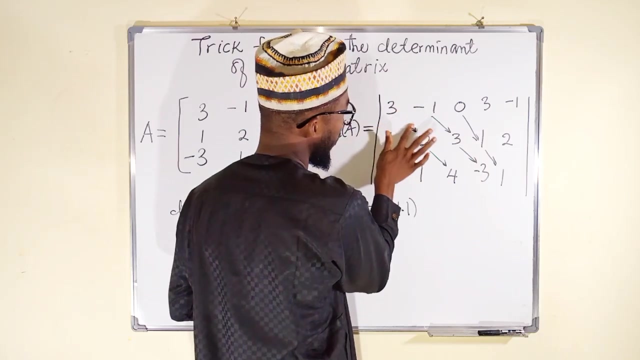 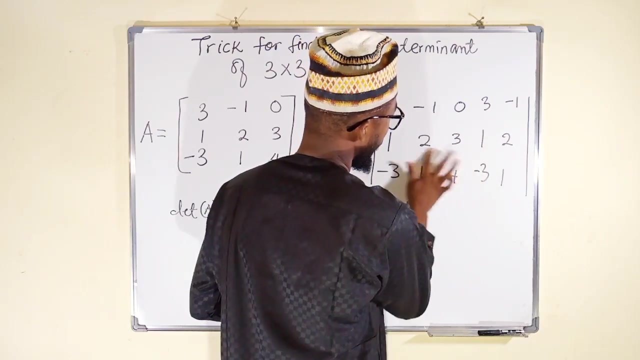 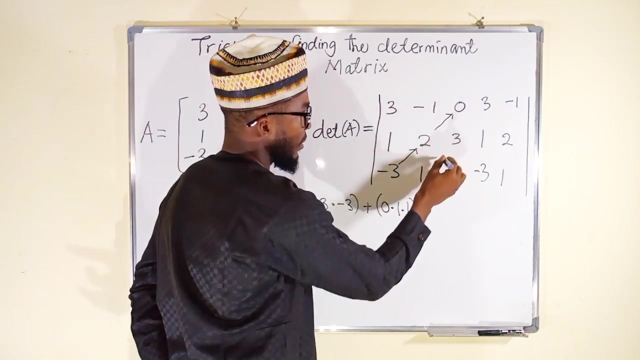 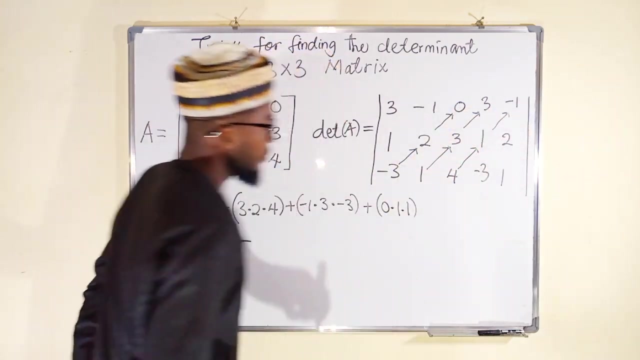 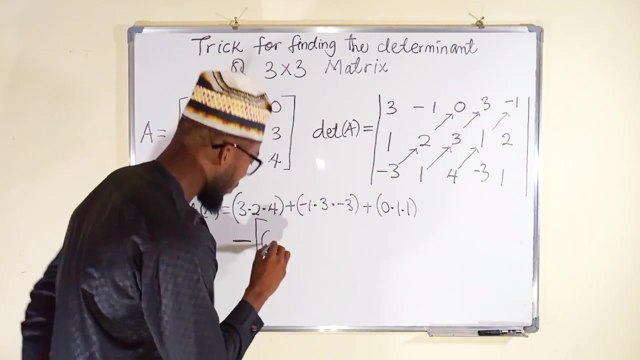 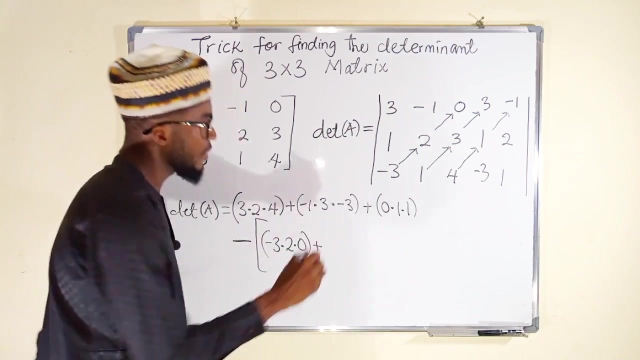 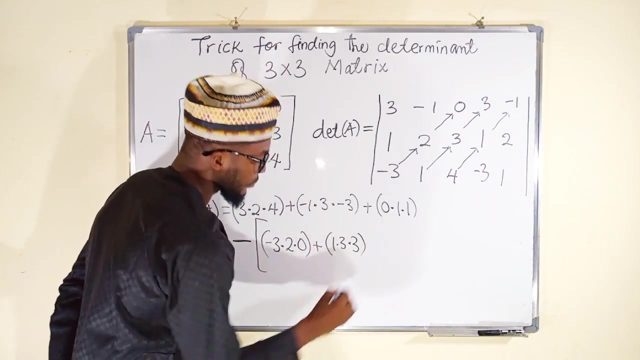 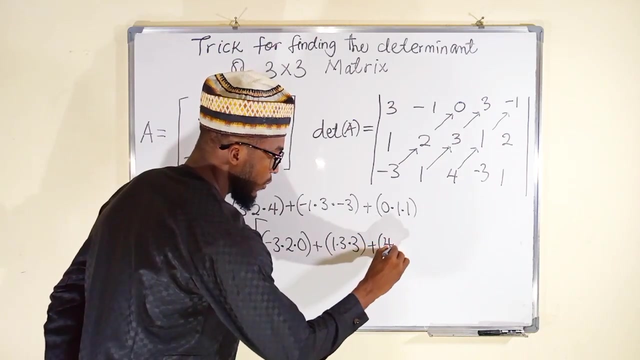 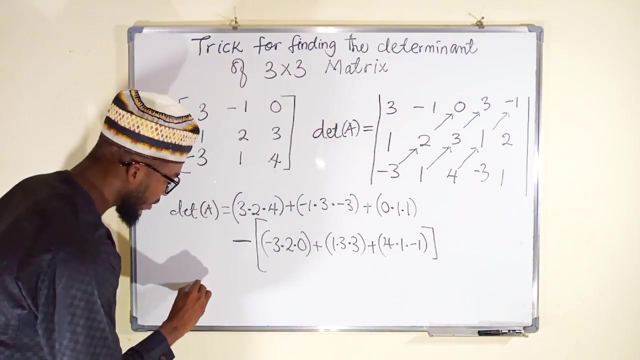 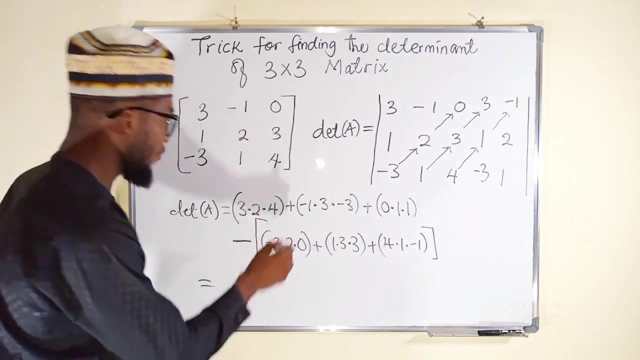 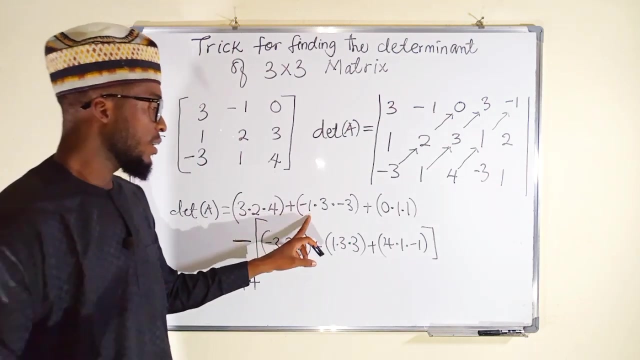 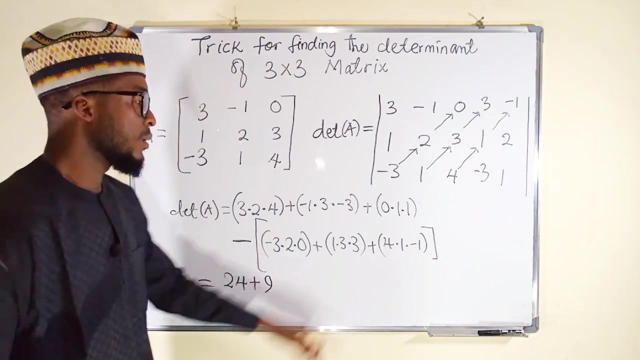 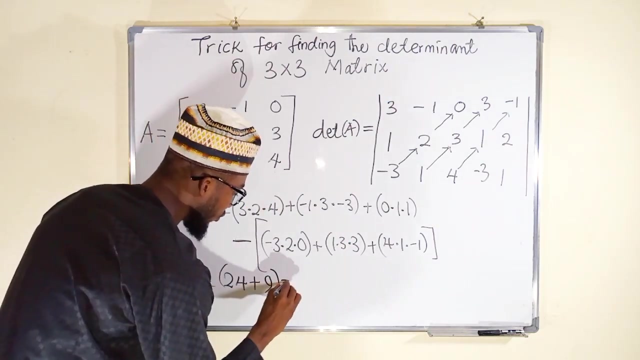 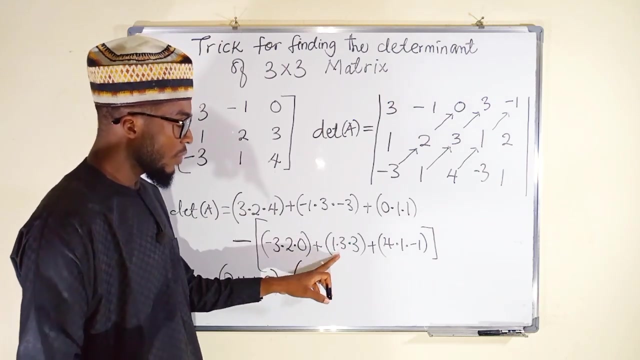 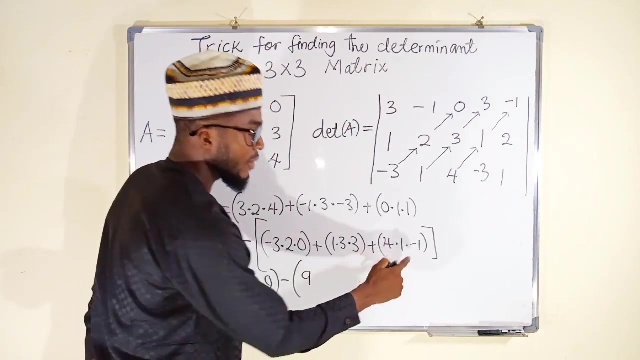 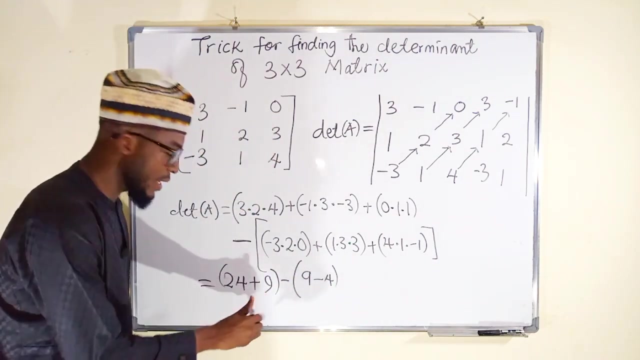 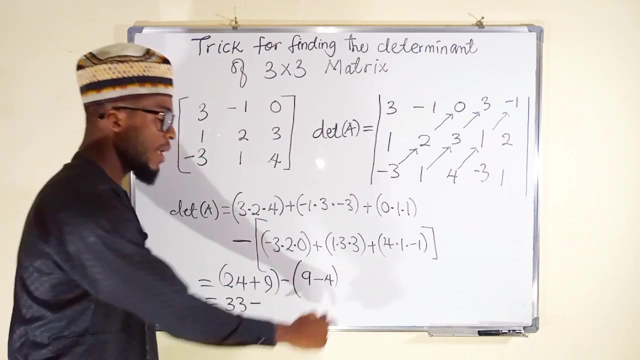 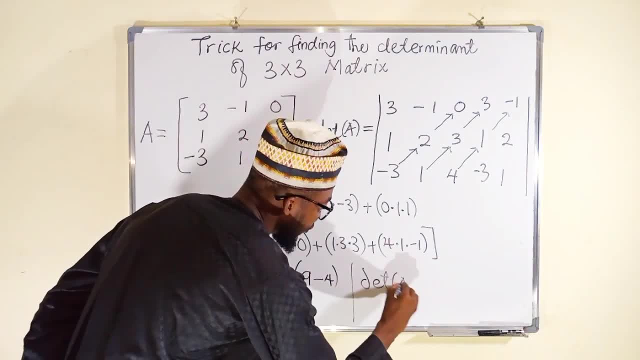 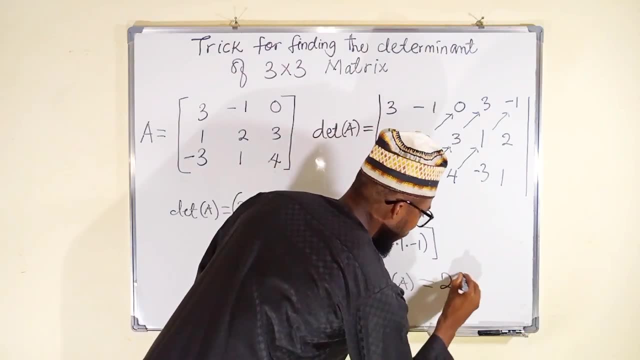 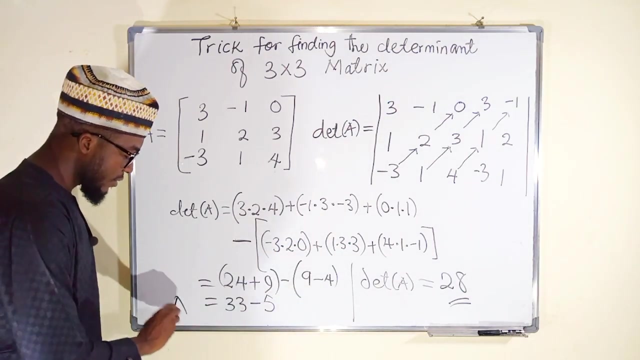 do it here determinant of this matrix a is going to be equal to 33 minus 5 which is equal to 28 and therefore the determinant of this matrix a is equal to 28 and this is our final answer and this is all I have 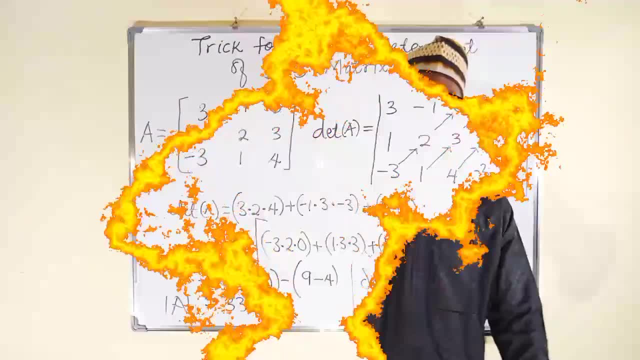 for you today thank you for watching do have a nice day